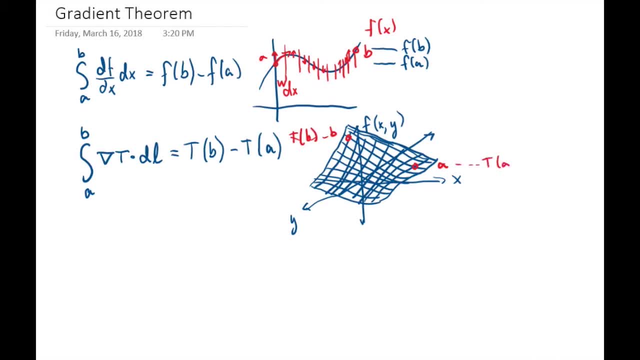 t of b and t of a, or we can look at the gradient along each infinitesimal part of the path and let's say we're taking like this path. so here it's flat, here it's flat, here it's flat, here it's this direction and uphill. 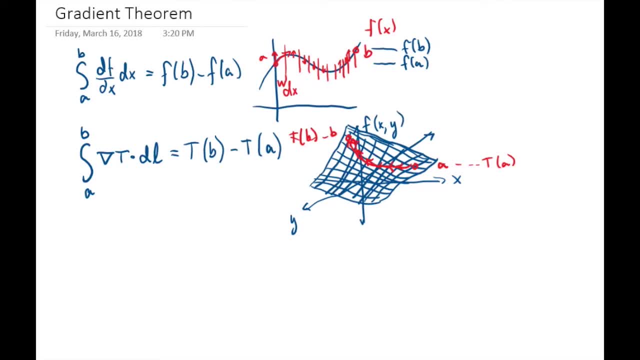 here it's this direction and uphill, here it's this direction and uphill. and all of these integrated together over the path will equal the total change in height. Now the divergence theorem, also known as Gauss's theorem and equivalent to Gauss's law for electricity, is a little bit harder to draw, but very intuitive. I'll try to do it. 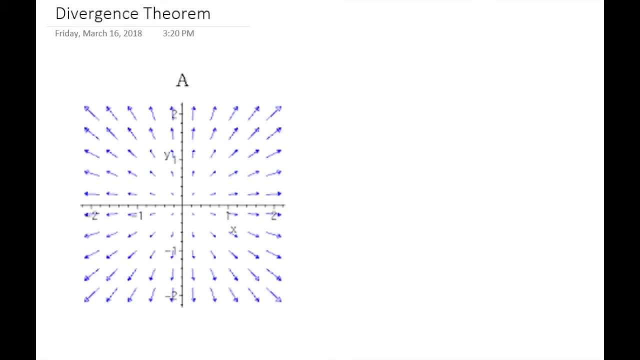 in two dimensions. So if we have some vector field, the divergence theorem states that the total divergence inside a surface- which in this case will be a one-dimensional line- but if it was a three-dimensional vector it would be a two-dimensional surface- The divergence inside, 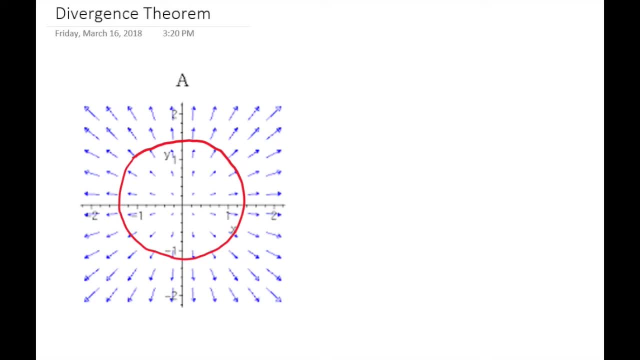 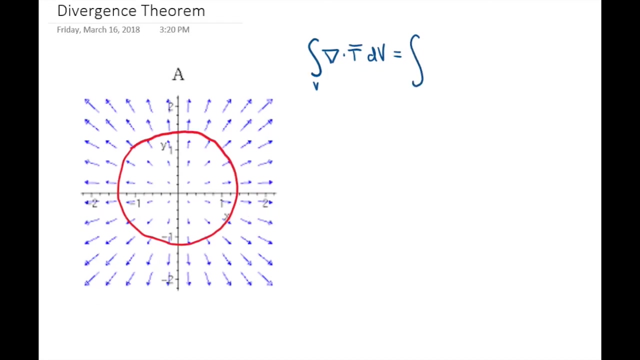 some closed surface is equivalent to the value of the function at the boundary of a particular tree of the surface and that will also be an integral. obviously, because the surface has area, We can write this as the volume integral of the divergence of the function over the volume is equal to the integral over a closed surface. the 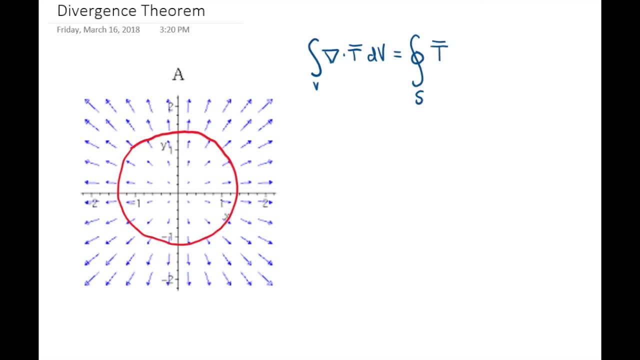 little circle means closed of the function itself, or DA is an infinitesimal piece of the surface. If we imagine that the vector function is some kind of fluid- for example, water flowing out of a faucet is a really good example- we're essentially saying that the amount of water flowing out of a 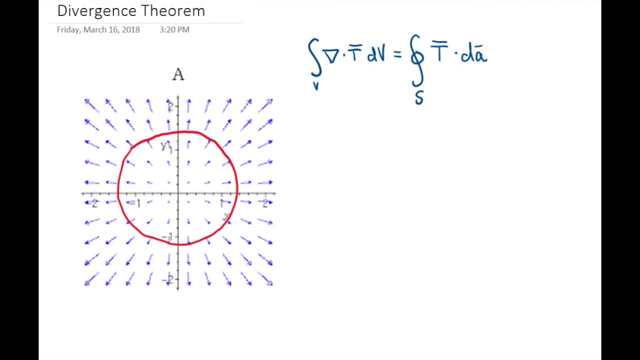 faucet into a pond has to be equivalent to the value of the flow of the water at the boundary of a pond, except in three dimensions. It's often very nice to choose a surface to use this theorem with that is symmetrical somehow with regard to the function itself. So, as you can see, 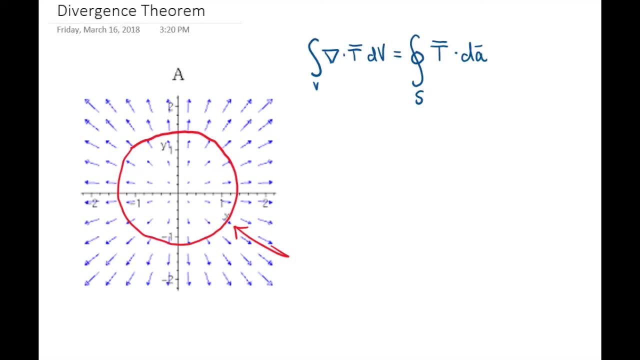 here I've drawn my circular boundary and the value of the function is actually going to be the same everywhere on this circle for the function drawn. so that's a really convenient way to write this, And this is used as Gauss's law in physics to solve a lot of problems. 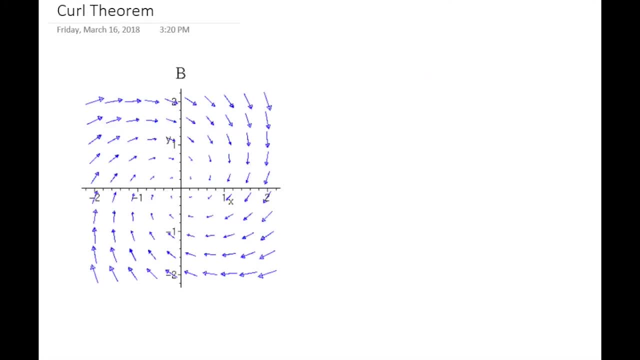 A fundamental theorem for curls, which is also known as Stokes theorem, relates the curl of a function over some area to its value at the boundary of the area. so this is a little less obvious, but it is easier to draw If I choose some closed line and we look at the curl. 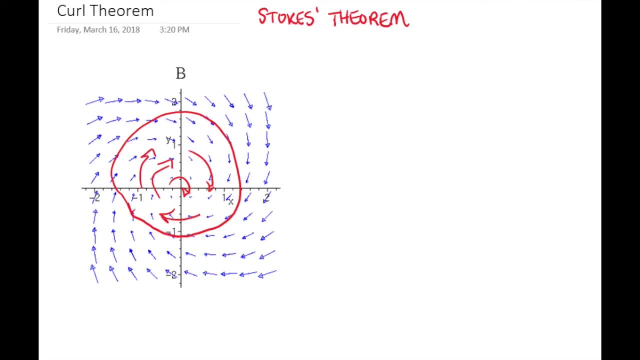 inside the line. the curl theorem, or stokes's theorem, says that by just integrating around the line we can find the total amount of curl inside the boundary, and the super cool thing about this is that it does not matter the shape of the surface at all. so in three dimensions we 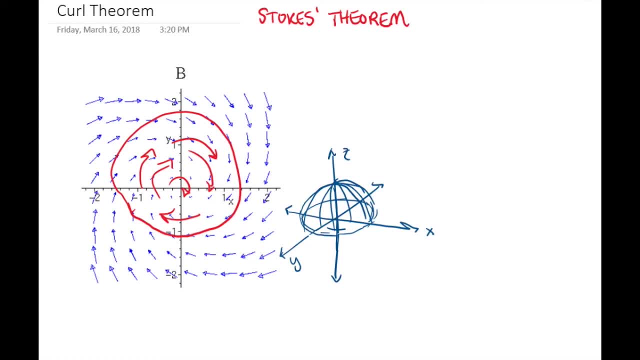 could have a surface that is, um, this terribly drawn hemisphere, and integrate along the boundary of it this bottom line. or we could have a surface that is just a flat circle, with the same boundary line, and stokes's theorem tells us that they will have the same amount of total curl. seems crazy. 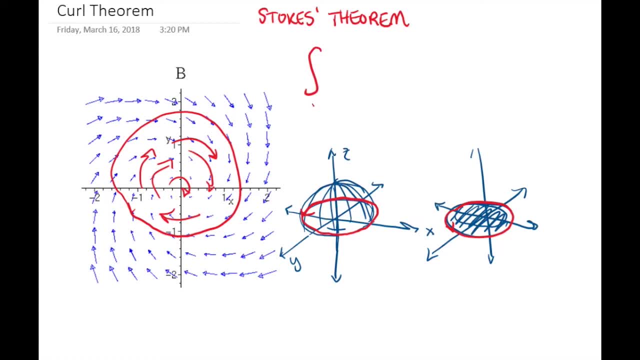 um. so the mathematical expression for this is the integral over a surface of the curl of the vector dotted with the area vector of the surface is equal to the integral around a closed path of the vector dotted with an infinitesimal piece of length. you'll notice that we didn't decide which. 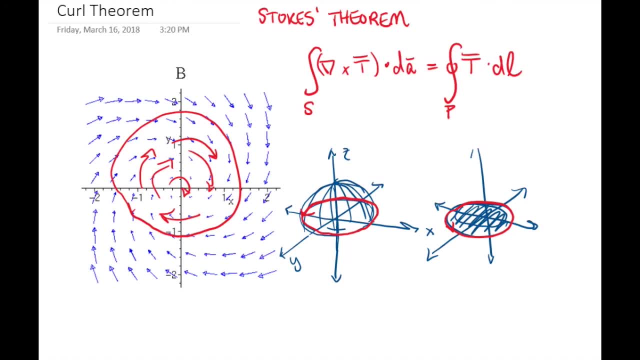 direction the area vector points. with a closed surface, it always points out, but with a non-closed surface it can point up or down on this surface. here, However, we also didn't determine whether the path we're integrating around goes clockwise or counterclockwise, And so we can just make sure.